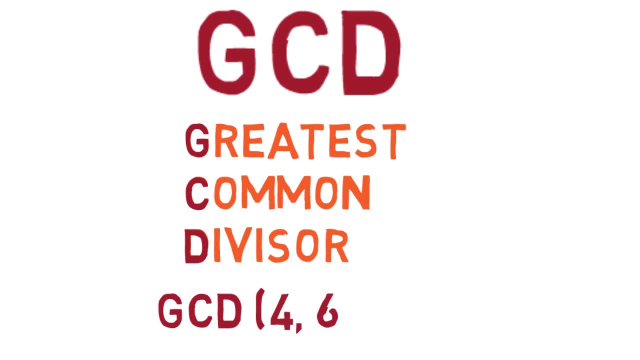 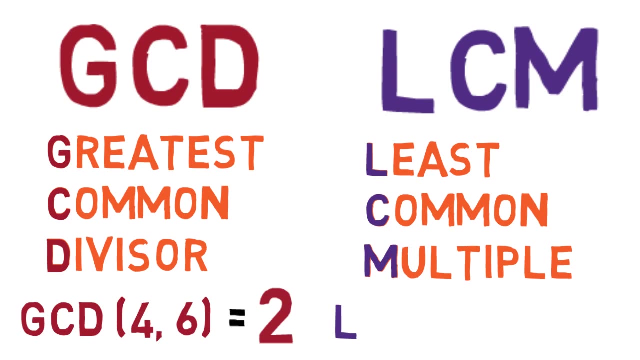 divisor. For example, the GCD of 4 and 6 is 2, because 2 is the greatest number. that's a factor of both 4 and 6.. In contrast, the LCM is the least common multiple. The LCM. 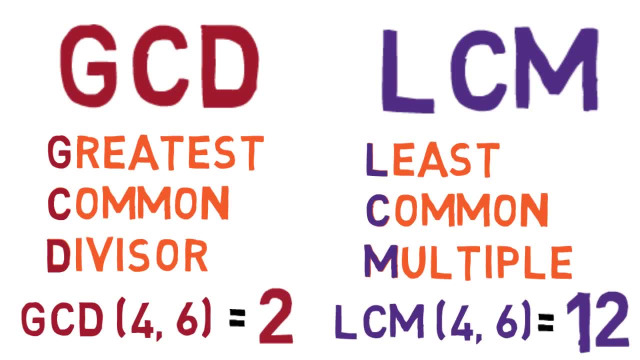 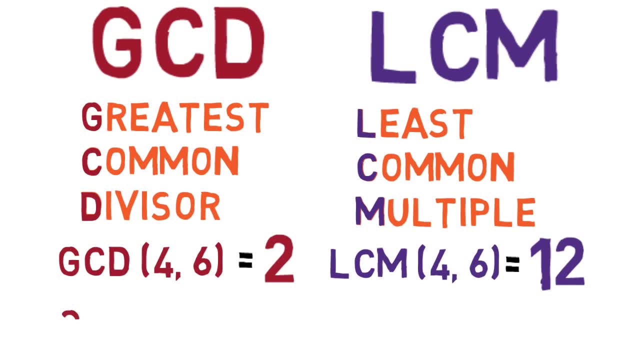 of 4 and 6 is 12, because 12 is the smallest number, that's a multiple of both 4 and 6.. As another example, the GCD of 6 is the greatest number, that's a factor of both 4 and 6.. 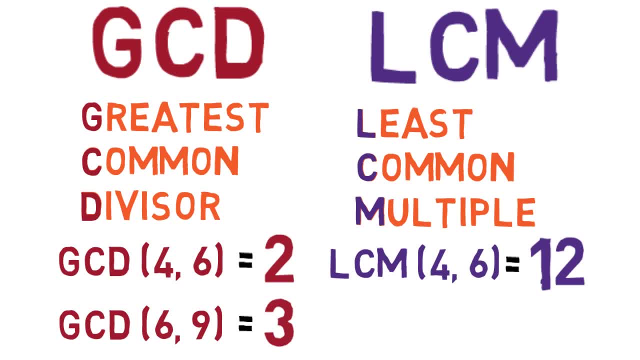 The GCD of 6 and 9 is 3, because 3 is the greatest number, that's a factor of both 6 and 9.. And the LCM of 6 and 9 is 18, because 18 is the smallest number, that's a multiple. 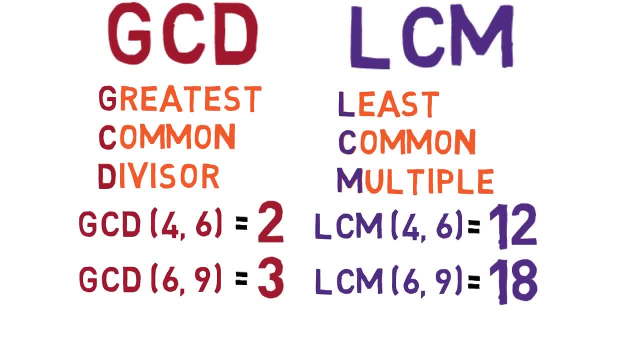 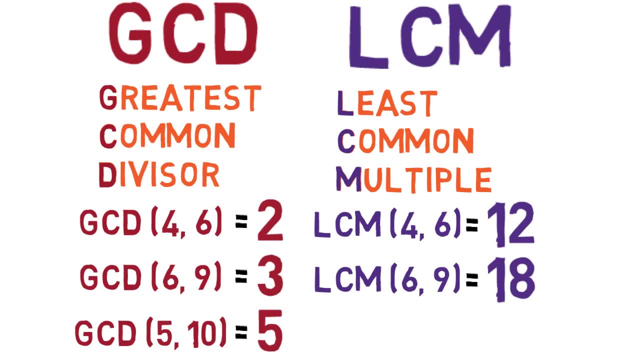 of both numbers. Here's one final example: What is the GCD of 5 and 10?? The answer is 5, because 5 is a factor of 10.. So it's the greatest common divisor of 5 and 10.. 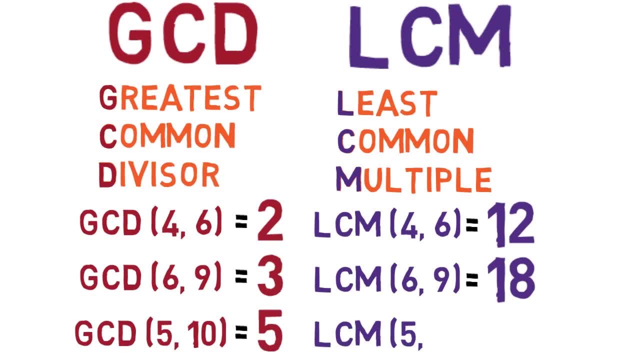 Now can you find the LCM of 5 and 10?? It's 10, because 10 is the smallest number, that's a multiple of both numbers. Notice that the GCD of 2 numbers is always less than or equal to the lower number, while the LCM is always greater than or equal to the greater number. 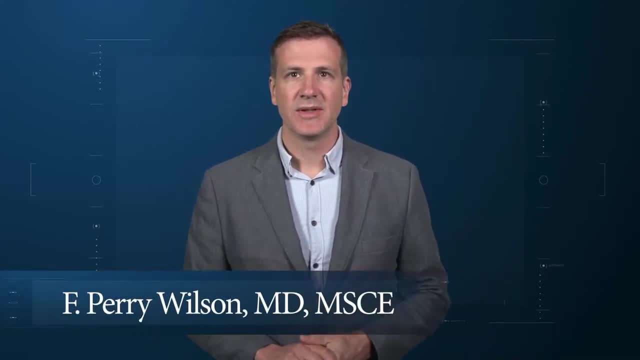 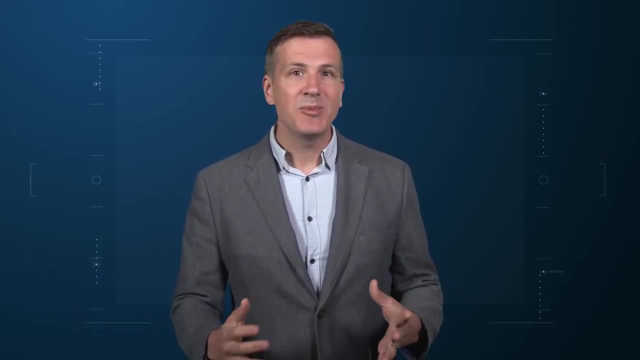 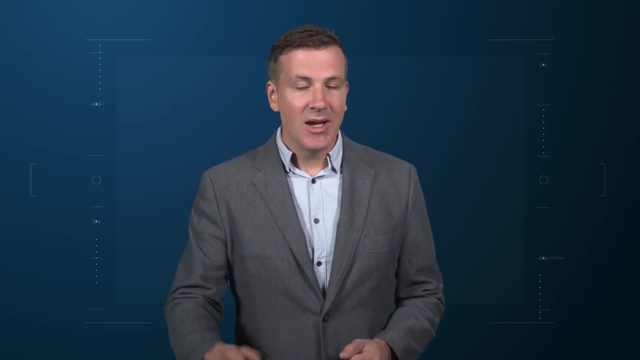 The idea of rationing medical care is anathema to most doctors. Sure, we acknowledge that the realities of healthcare costs and insurance companies might limit our options, but there's always a sense that when something is truly, truly needed, we can get it done, Except in one very particular situation, a situation where rationing of care is the norm. That situation: Organ transplantation. There is no way around this. More patients need organ transplants than there are organs available to transplant. It is cold hard arithmetic. No amount of negotiating with an insurance company, no amount of engaging in prior authorization. 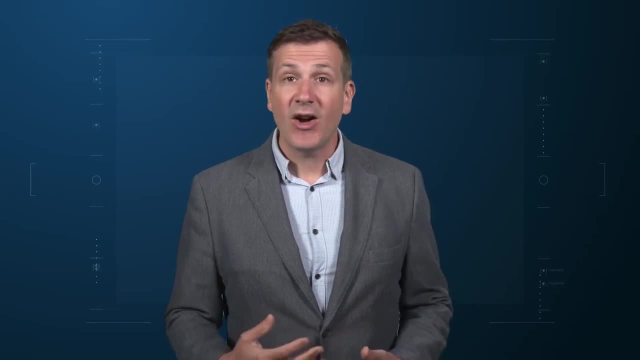 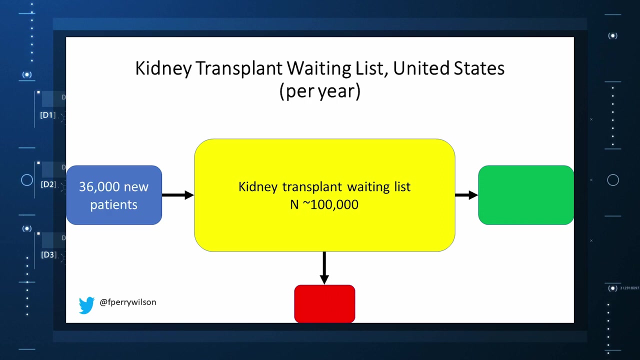 can change that. As a kidney doctor, this issue is close to my heart. There are around 100,000 people on the kidney transplant waiting list in the US, with 3,000 new patients being added per month. There are only 25,000 kidney transplants per year and each year.